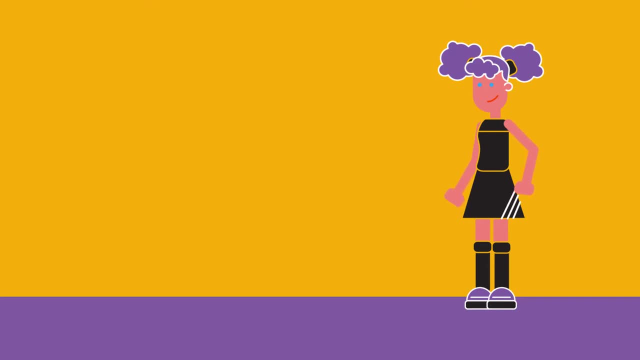 Because the ball is slowing down, we can say that its velocity is changing. By Newton's first law, this means that the ball is experiencing an unbalanced force. In this case, it's the force of friction that opposes the motion and eventually stops the ball. 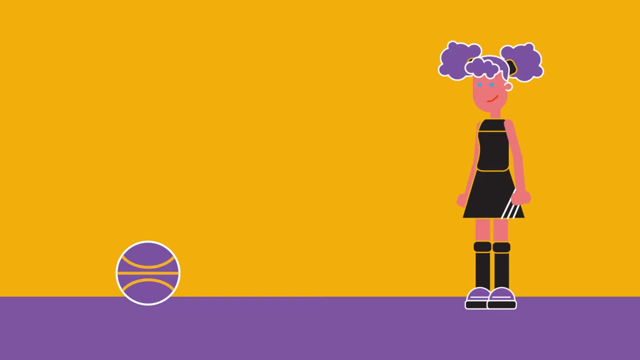 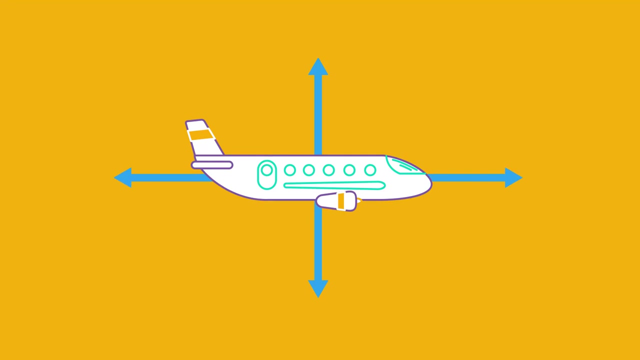 Note that there is no forward force on the ball. She is no longer kicking the ball, so there is only backward frictional forces which slow the ball to a stop. Look at the diagram of the aeroplane shown. If the thrust of the engines is equal to the 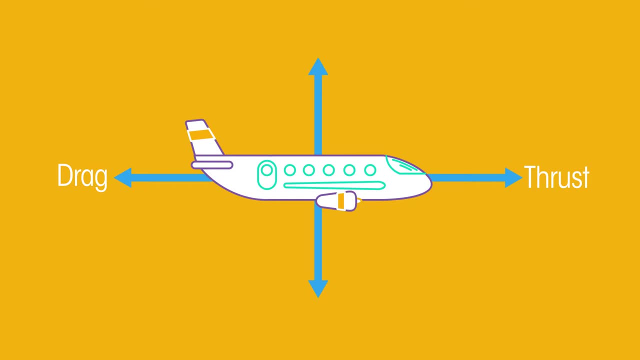 drag force, it will move forward at a constant speed. The plane will travel at constant height. if its weight is balanced by the lift force from the wings, We have uniform motion. If the plane wants to move faster and increase its velocity, then the thrust force pushing the 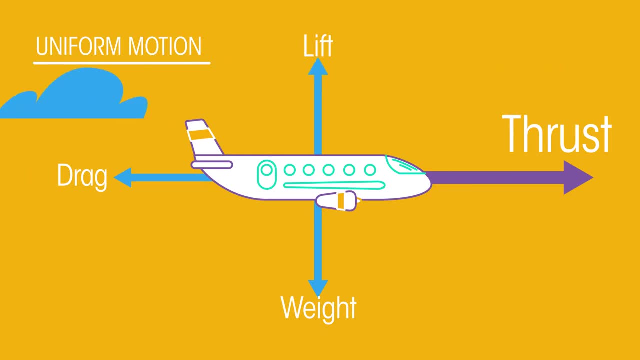 plane forward needs to increase. It becomes larger than the force of air resistance and creates an unbalanced net force. The plane now accelerates, no longer moving with uniform motion. Drag increases with velocity. so very soon the plane will have balanced but larger forces again and its velocity remains constant, but higher than before. 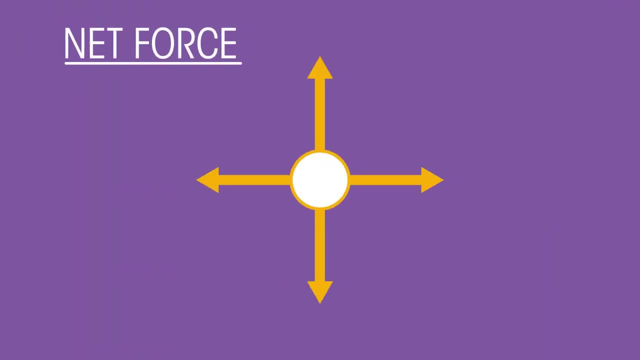 Quantitatively, we can find the net force of any object by considering the size or magnitude and the direction of each force acting on an object. It can helped to draw on the forces yourself. Take a look at this example here, which shows three forces acting on the object. 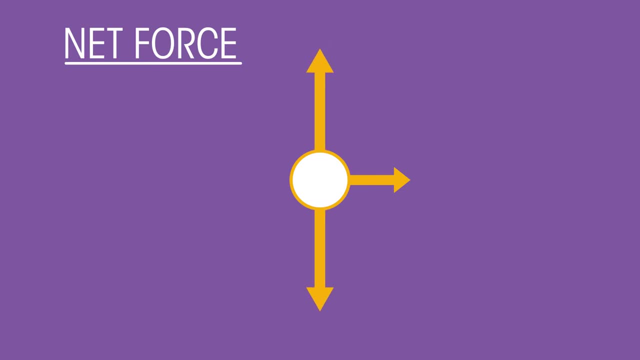 The two vertical forces are equal and opposite, therefore cancelling each other out. However, the horizontal force has no opposition, and so it remains unbalanced. This means that the net force will act to the right and will have the magnitude of the horizontal force. 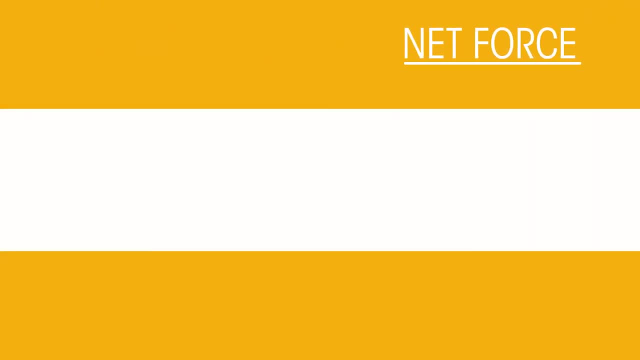 When working out the net force, it's a good idea to consider the horizontal and vertical directions separately. At the end these directions can be added up to give you a diagonal force. You can think of these forces to be a bit like points on a compass.